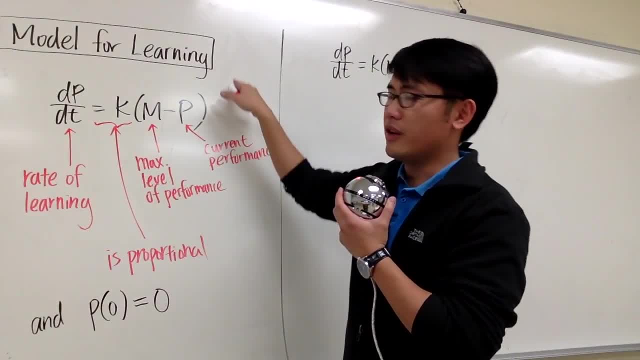 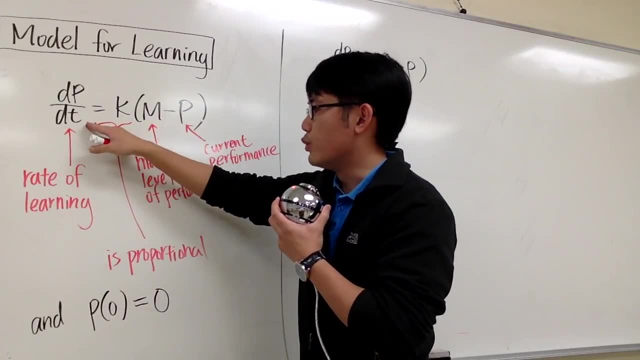 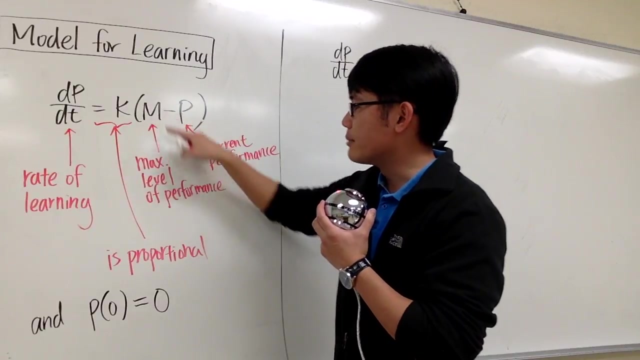 Let's take a look at this differential equation, which is a model for learning and which says: dp. dt equals to k times m minus p. In words, I can say this as the rate of learning- how fast a person can learn- is proportional to the difference between the maximum level of performance somebody can ever achieve and the current performance that the person is at right now. 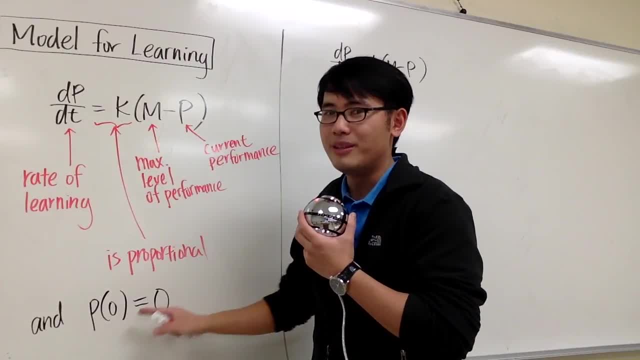 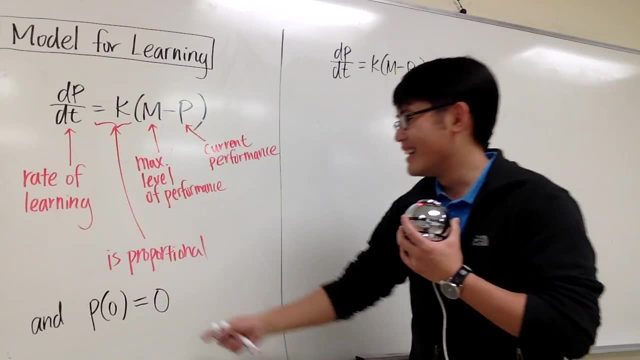 And we also have an initial condition: p of 0 shall be 0. Why? Because before we learn anything, certain skills or so we don't know anything about it. That's why the performance will be 0, at times equal to 0 before you learn anything. 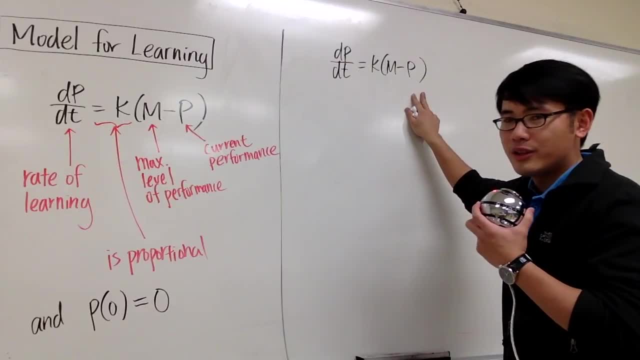 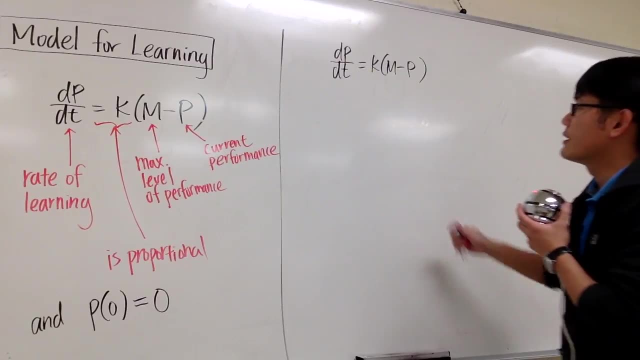 Anyways, our goal is to solve this differential equation and also we have to use that initial condition and we'll also take a look at what's the limit of p of t. As you can see, this is a separable differential equation. 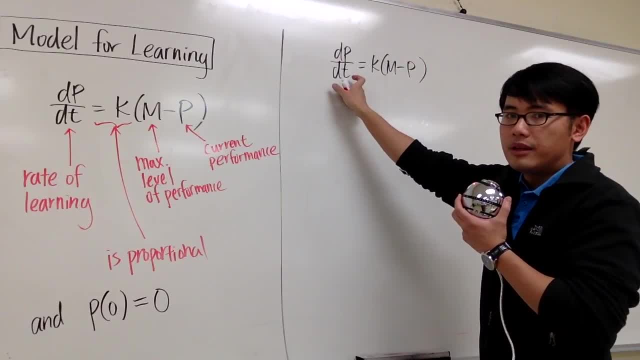 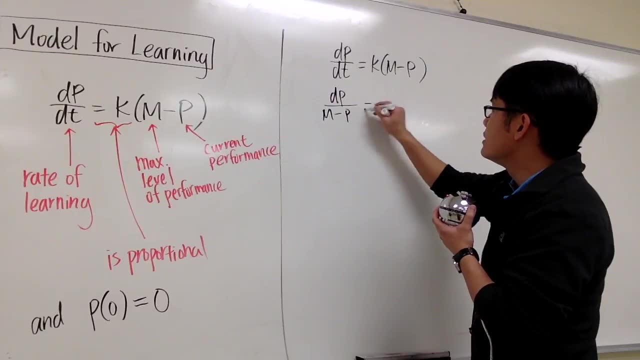 I'm going to bring this factor down to the denominator and I'll bring the dt to the right-hand side, So it will look like we have dp over m minus p. this is equal to k times dt and then, with that being said, we can integrate both sides. 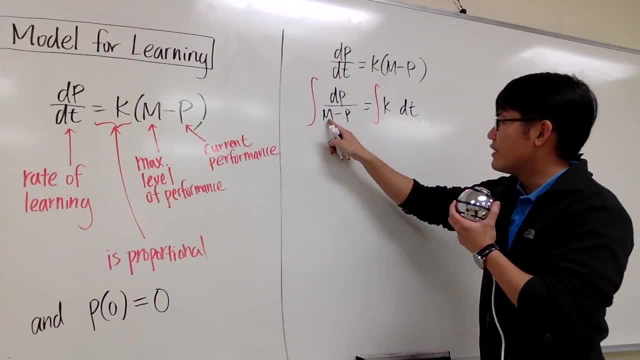 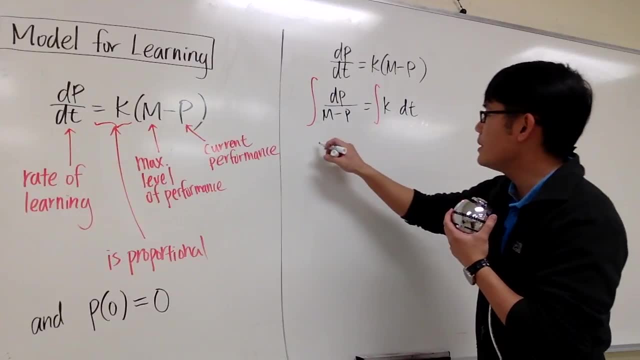 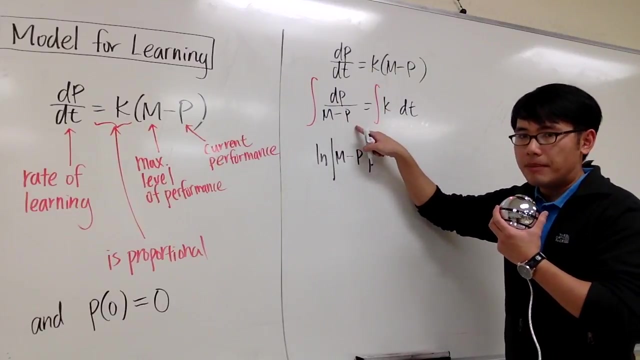 So integrate here. integrate here. Notice that we have a linear factor on the denominator. so this is linear factor in terms of p in the denominator. The antiderivative of this is just going to be ln, absolute value, m minus p. But then the derivative of m minus p is negative. 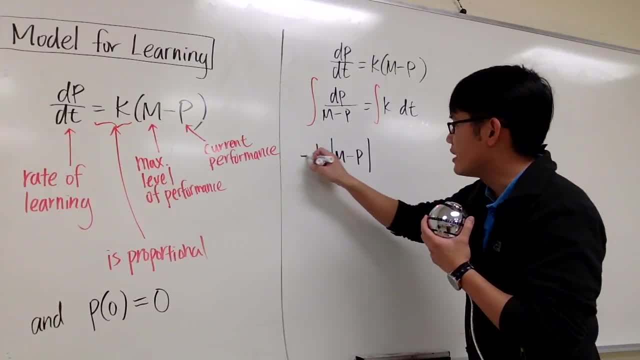 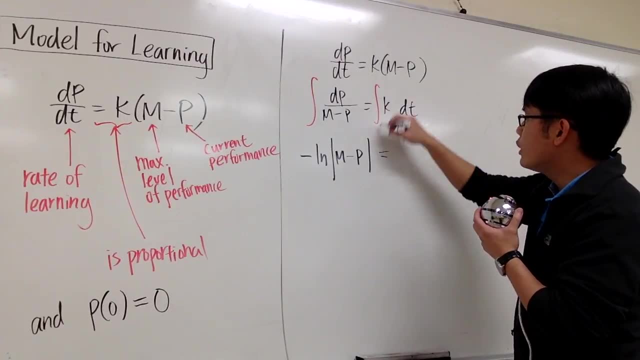 So we have to divide it by negative 1, so we need a negative right here. You can also do U-sub, but this is going to be the result, And this is equal to integral of k. in the t-world is kt, and then we have to have a constant. 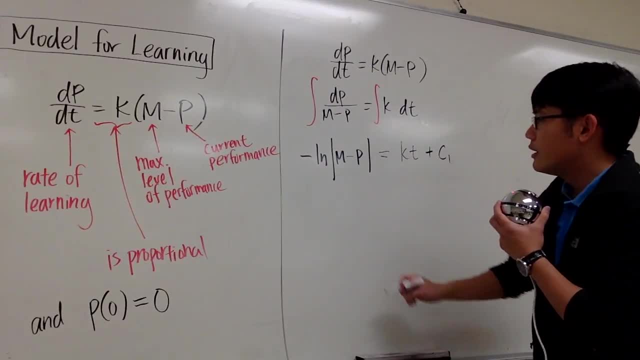 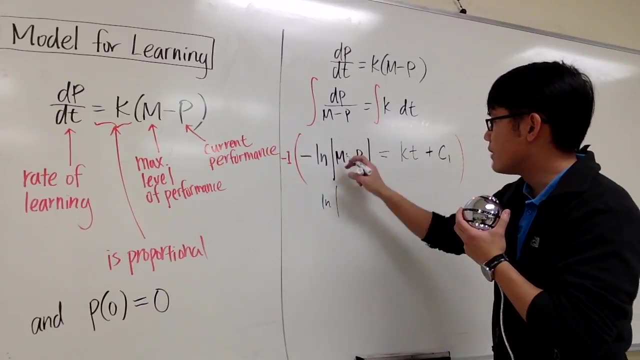 So that's my first constant. I'll call that c1.. Alright, so let's multiply everything by negative 1, so I can get rid of this negative And I will have ln absolute value, m minus p, And this will be. 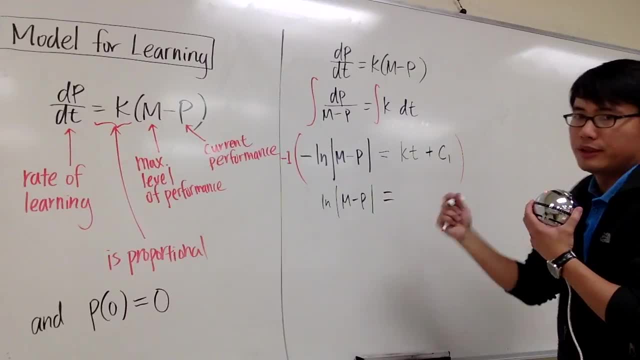 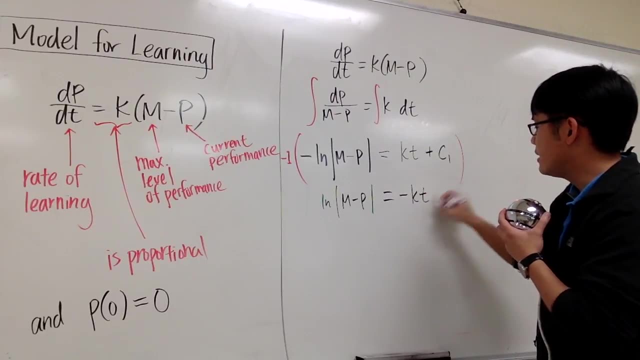 Negative 1 times kt. Well, k is preset, so I'm not going to call that a k2 or something. I'm just going to put this as negative kt, But then negative 1 times c1, I have the right to make that into a c2.. 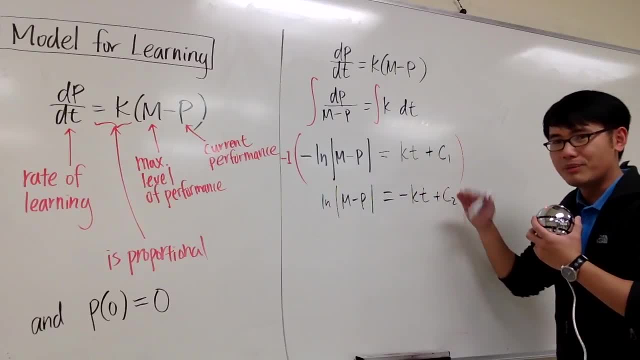 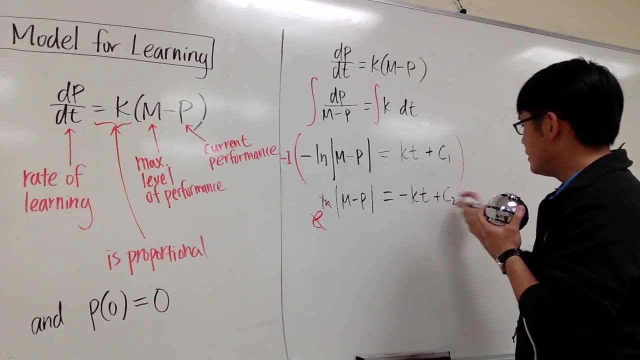 So I'll just put that plus c2.. But technically it's minus c1,. but this is okay. Alright, to get rid of the ln. I will do e to the power so they cancel. I'll pretend this is my exponent and then I'll do e to the power. 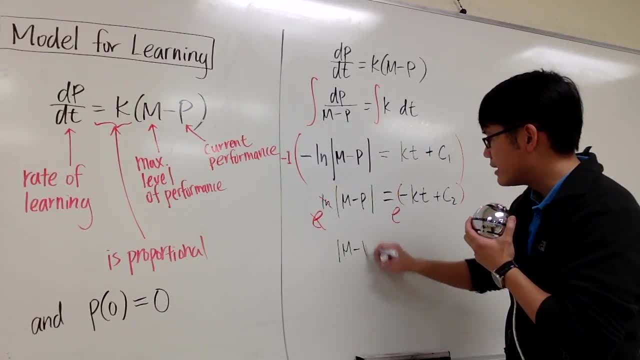 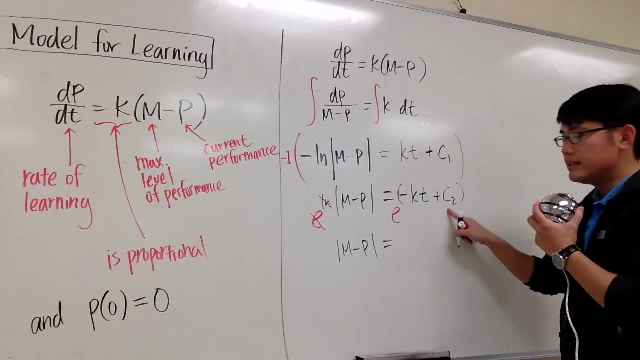 On the left-hand side, I will have absolute value m minus p, And this is equal to Well, if you take a look at this, we have two things that's been added in the exponent And this is technically saying: let me just put this down on the board. 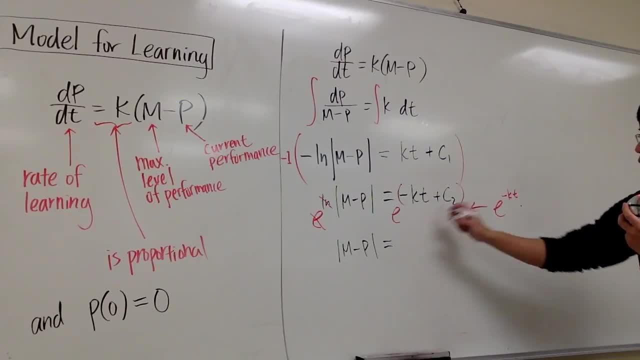 e to the negative kt, times e to the c2.. Right, Because when you multiply two things that have the same base, we just need to add the exponents, And when you're adding the exponents, we can break it apart into two things multiplying have the same base. 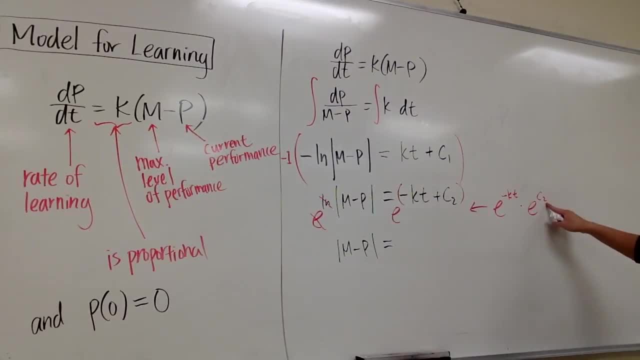 This is the function part. I cannot change it. But then when we have e to the c2, e is a constant, c2 is also a constant. we can call that just another constant, say that's c3. And then this is e to the negative kt. 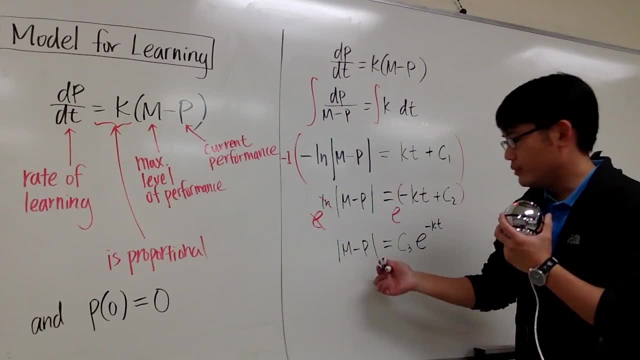 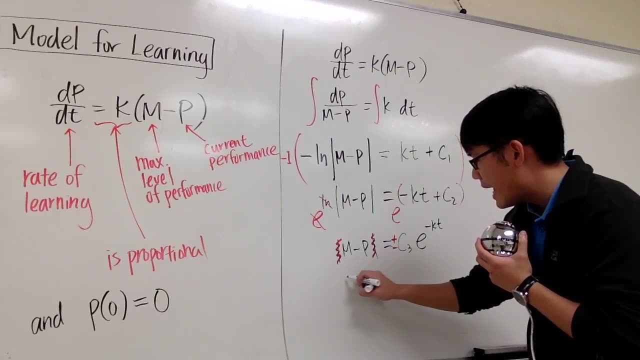 Okay, Alright, I need to get rid of the absolute value. so I can just say, alright, let me get rid of this absolute value, and then I'll put a plus- minus on the right-hand side, And then we will have m. 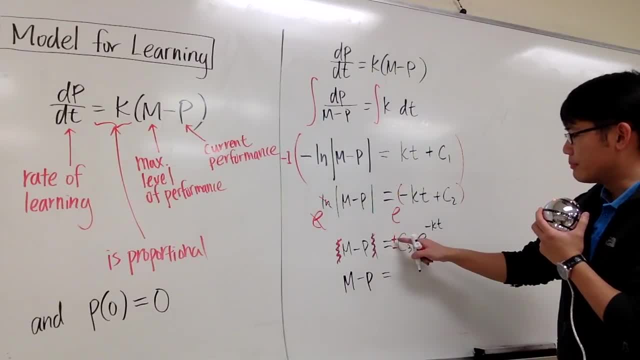 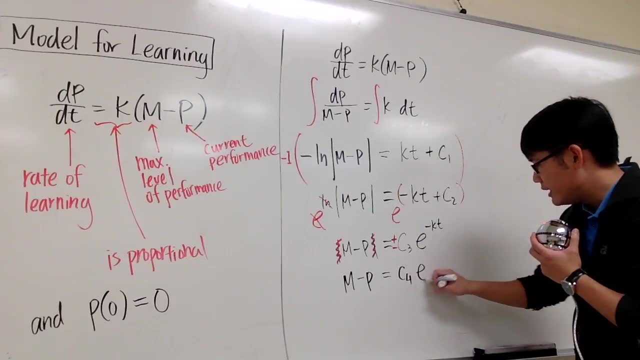 Minus p equals to well, I don't know if it's plus or minus c3.. I'm just going to call that another constant. so keep track. This will be my c4.. And we have e to the negative kt. 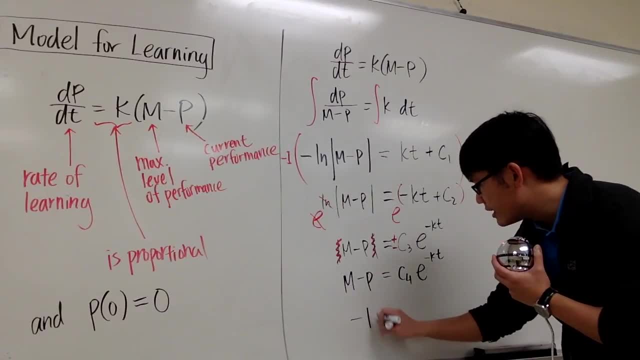 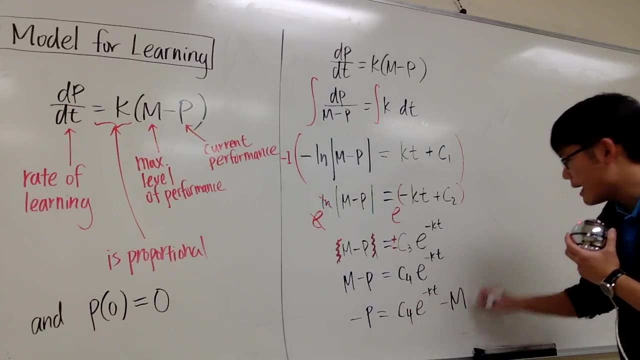 And I just need to subtract m on both sides. I get negative p equals to c4 e, to the negative kt minus m. And the last touch is that I need to isolate this p. I will multiply everything. I will multiply everything by negative 1.. 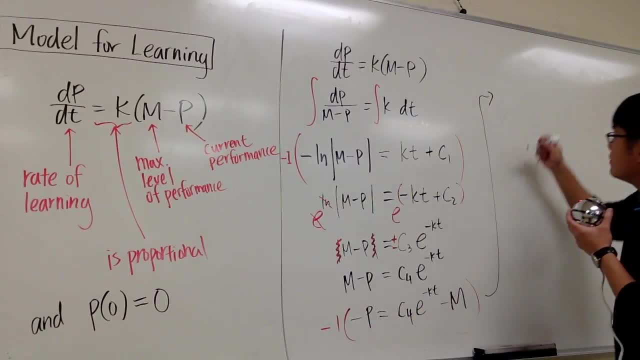 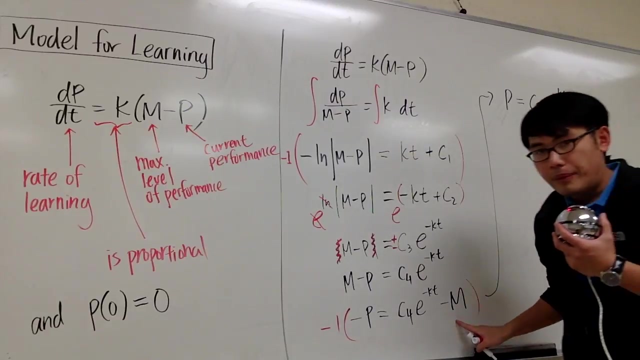 So, as you can see, we will end up with positive p And this will be negative 1 times c4, which is like c5.. I'll just say that c5 e to the negative kt, But m was preset, so we will have to keep it as m. 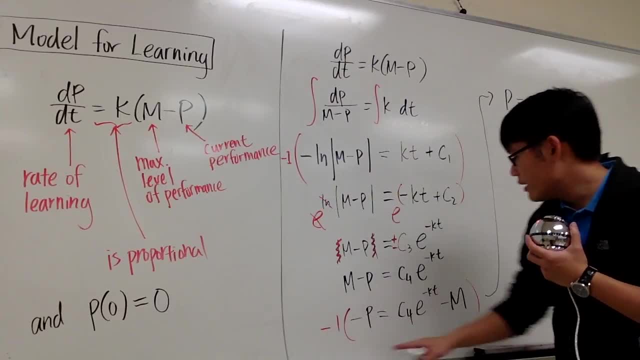 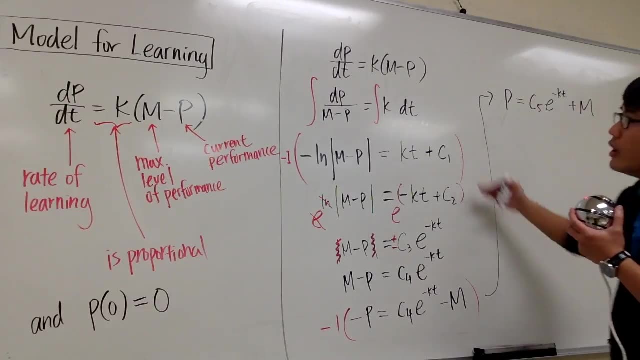 I cannot call that m2 or anything. I will just write it as negative 1 times negative m, which is plus m. And I'm done, Because this is the general solution to this differential equation. And now let me just kind of write it legitimately. 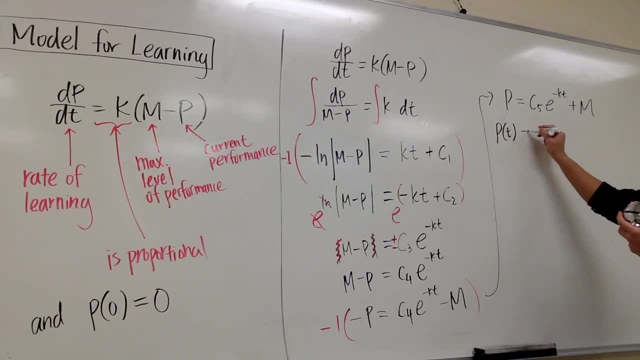 This is p, which is a function of t. It's equal to some constant c- I don't know yet, so I will just call that c. So let my c for the answer, e to the negative kt and m plus m. 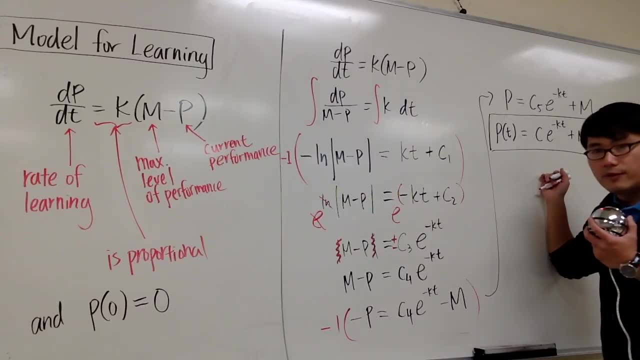 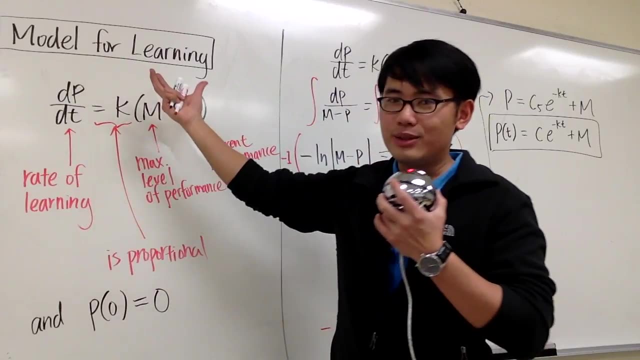 This right here will be the general solution to my differential equation. But then I do have an initial condition: At first I don't know anything. If I use this to model how a person learns Before we learn that skills, we don't know about anything. 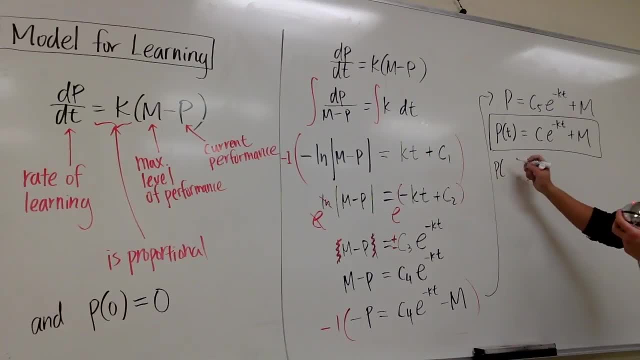 All right, So I will just plug in, let's say p of 0. This will be 0.. I will plug in 0 into this. t We get c e to the negative k times 0 plus m. We'll solve this equation. 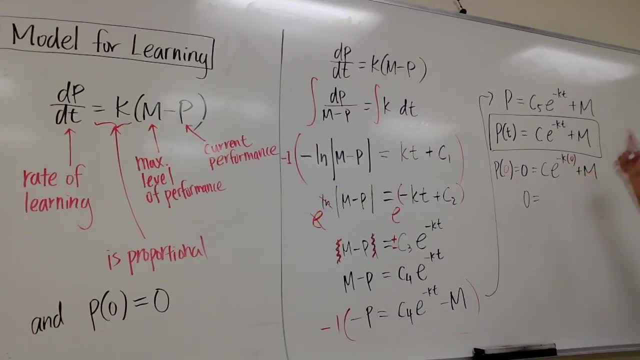 This is 0, equals to e. to the 0, power is 1.. So we have c, So we have e to the negative kt plus m. In other words, I can say c is equal to bring the m to the other side, which is minus m. 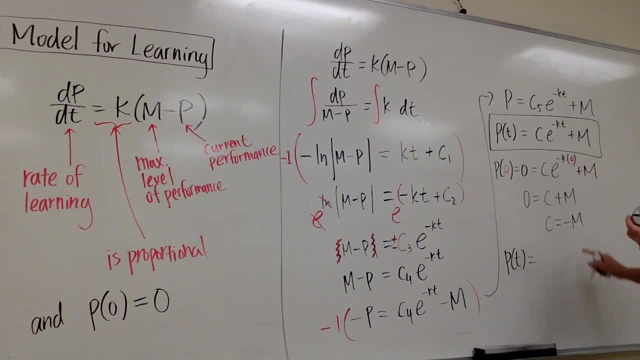 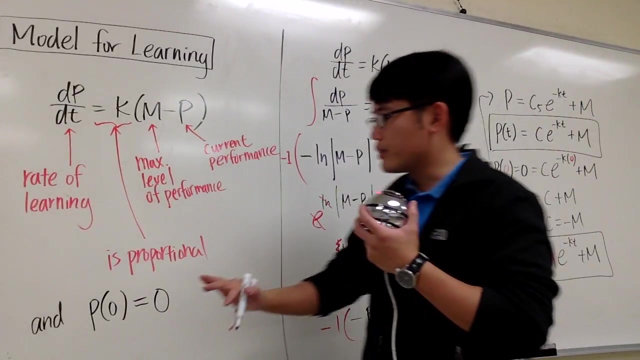 And therefore p of t is going to be negative m for the c-value e to the negative kt plus m. So this right here will be pretty much the specific solution, the particular solution based on this initial condition, And also we like to take a look. 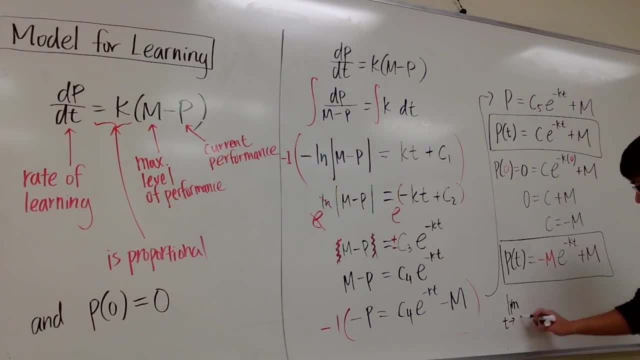 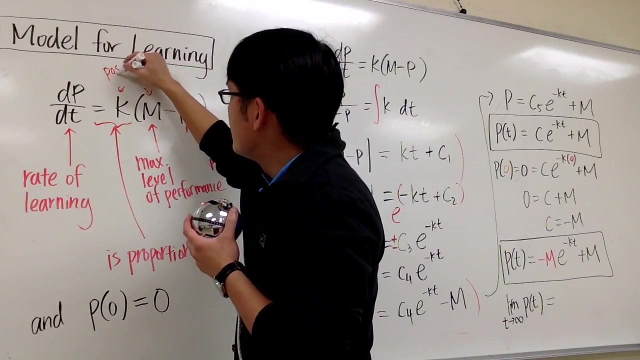 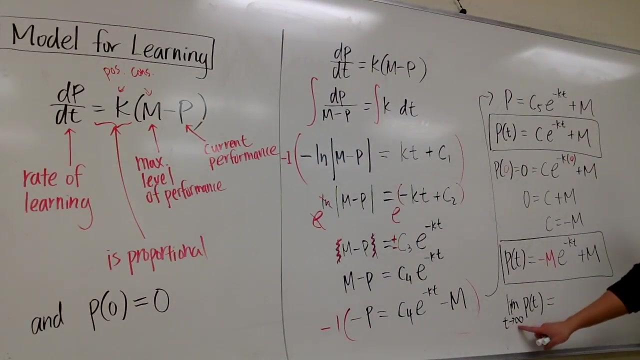 What happens if we take the limit as t goes to infinity of my learning curve, Okay? Well, first of all I should have come back here. This k and this m- in fact they are both positive constants. Okay, So if we have t is approaching infinity, we plug it into here. 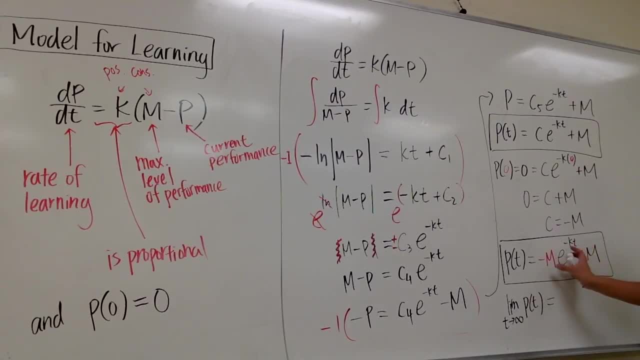 e to the, technically we will have negative infinity. This term will go to 0. And the only thing left is m. So we will just have the m, And you see that this right here was saying that the limit as t goes to infinity, our performance is equal to m. 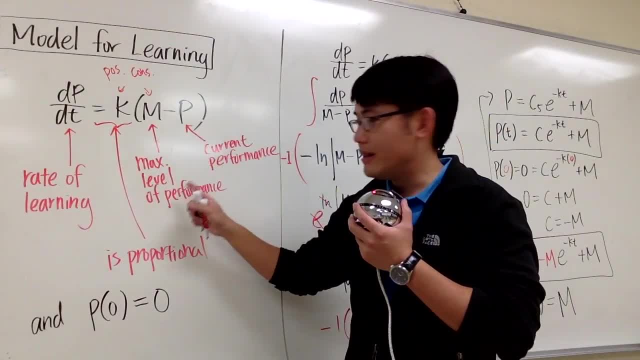 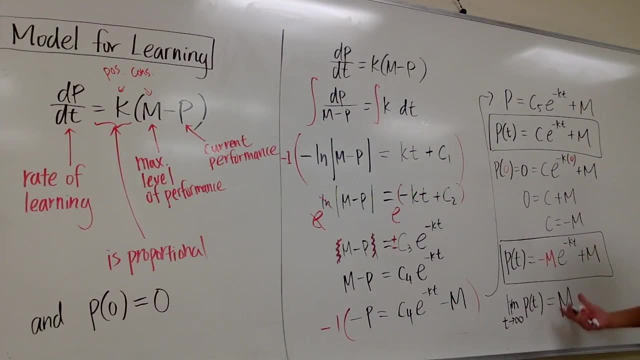 And what's m? And that's exactly our maximum level of performance. So it makes total sense, right? It makes perfect sense that at the end I will reach my maximum level of how well I can do a certain skills. So this is it.